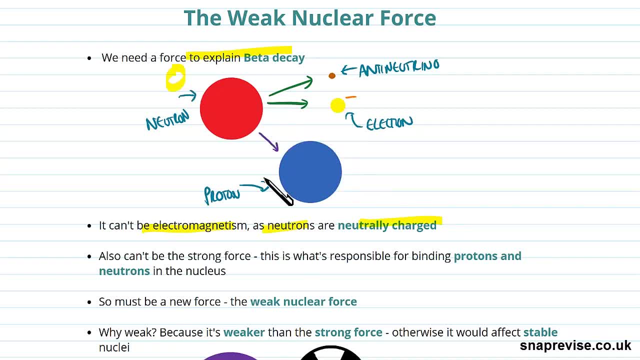 of zero. so how is it what's going on here? It can't be that It also can't be the strong force, because we know what the strong force does: It's what's responsible for binding protons and neutrons in the nucleus. It can't also be making neutrons decay into protons. 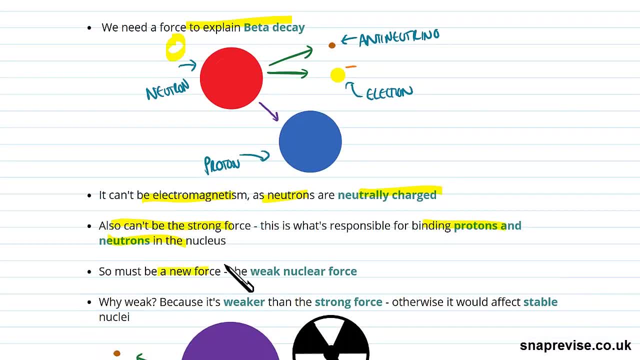 or whatever. It can't be that. So it must be a new force that we call the weak nuclear force. Why do we call it the weak nuclear force? Because it's the weak nuclear force. Why do we call it the weak nuclear force? Because it's the weak nuclear force. Why do we call? 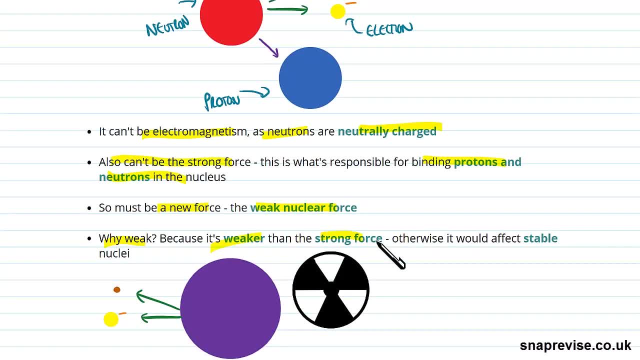 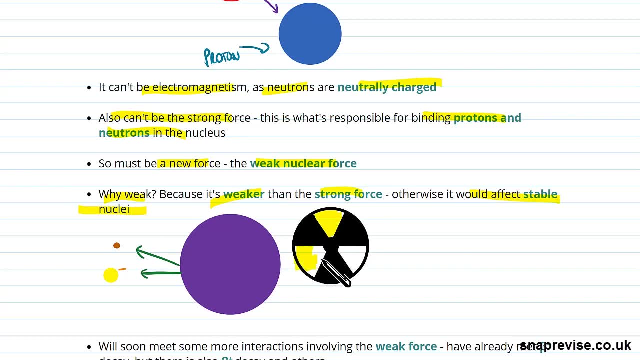 it the weak nuclear force? Because it's the weak nuclear force, Why do we call it the N sponsors? strong nuclear force has to be, otherwise it would affect stable nuclei. It only works if we've got these radioactive particles. They decay. If the weak force was stronger than the strong nuclear force than any particle always would decay, Whereas, as it is, only affects particles with unstable nuclei, and that's what gives us this beta k. This was our unstable nucleus then. that's what deристmann's unpaired nucleus And that's what deraszamです. 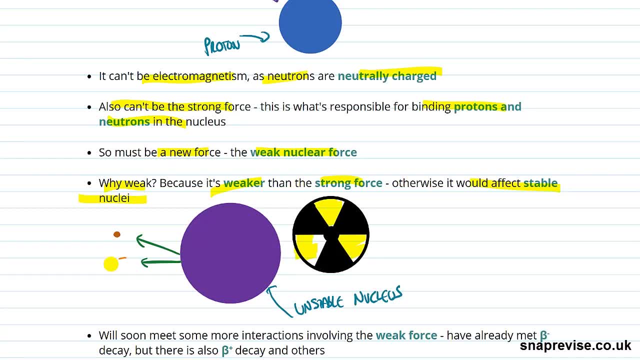 decays and actually what we have happening in here is a neutron changing into a proton. obviously we can't see that because we're at the scale of looking at a huge nucleus like i couldn't possibly draw so many protons and neutrons together. but the idea is that somewhere in here a neutron is. 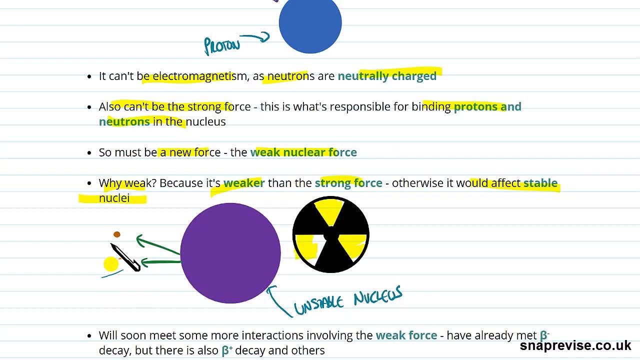 changing into a proton and that's what's emitting this, this beta minus particle, and this, this anti-neutrino. but that only happens for for radioactive particles, right, it only happens for unstable nuclei. it certainly doesn't happen for all nuclei, otherwise the world would be a 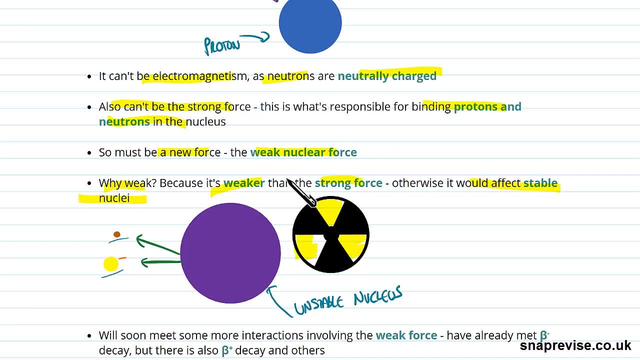 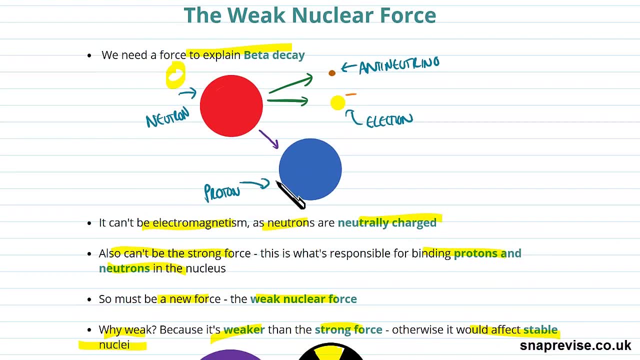 very different place, um, and so that that's what means it's weaker than the strong force. and it turns out there are many, many weak interactions. so we just literally look to one here: beta minus decay of a neutron into a proton. but there's many more and we're soon. 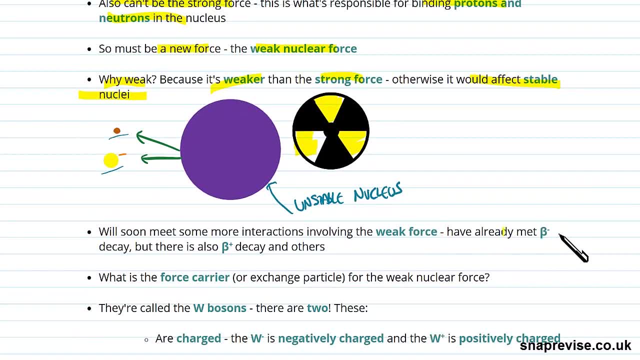 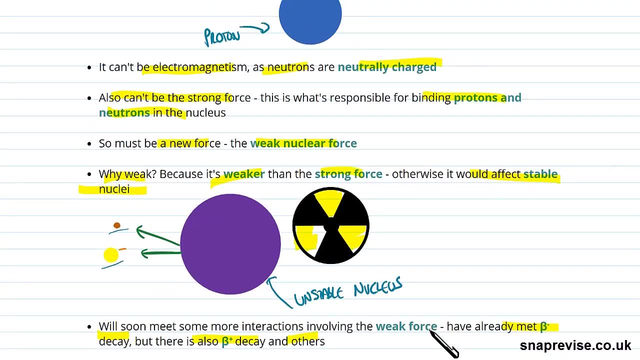 going to meet, uh some more. for instance, uh beta. we've seen beta minus decay, but there's also beta plus decay, so positron, decay and others. um, so we we're okay with the idea that forces- or at least we've seen one example, uh electromagnetism here, where there is an exchange particle, this virtual 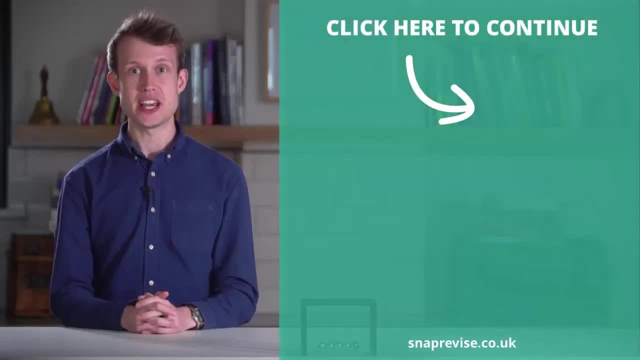 photon. hey guys, to continue watching this video and unlock hundreds of other super concise and exam board specific a-level physics videos, just click the snap. revise smiley face. join me today and together let's make a-level physics a walk in the park.